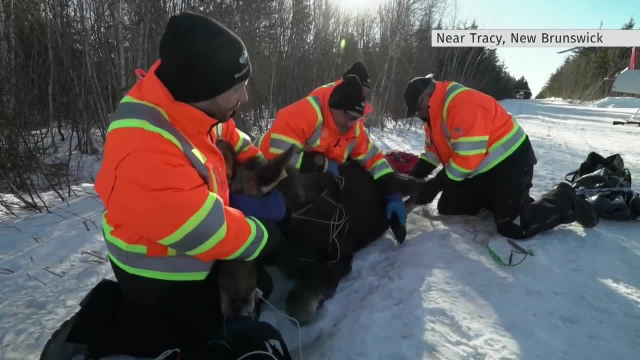 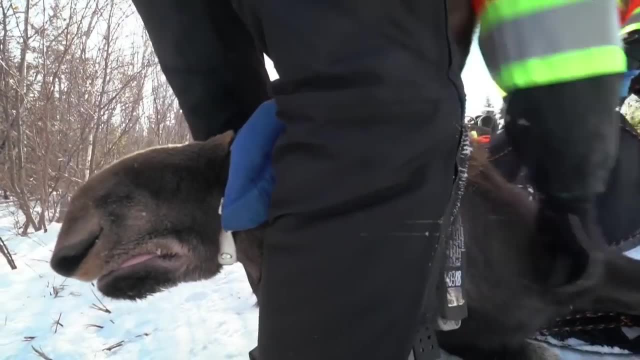 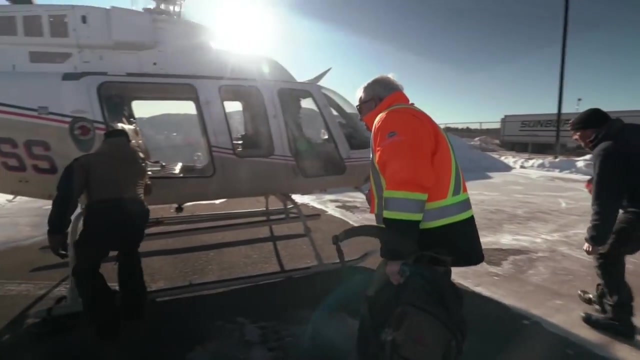 They swoop in like a pit crew, A team of scientists working quickly and efficiently to get what they need from the moose, All in an effort to help the species. The researchers from the universities of New Brunswick and Laval are determined to make sure. 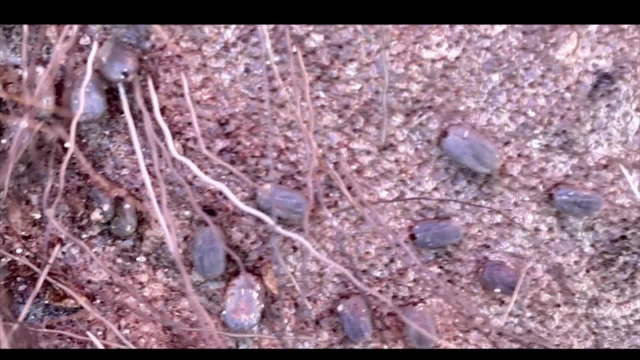 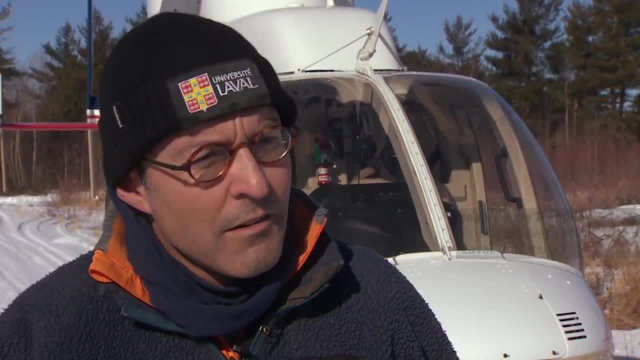 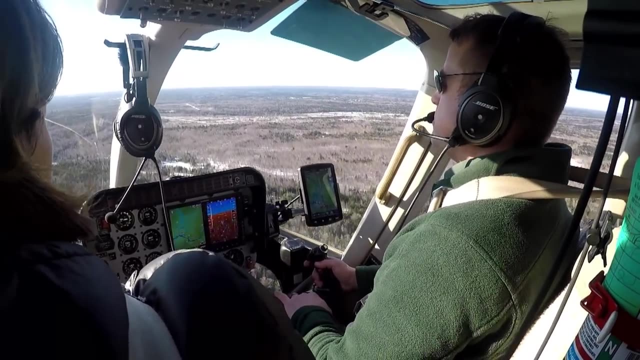 moose aren't wiped out by these tiny blood-sucking parasites, Winter ticks. They're an external parasite. They eat on their blood and they will stay there all for the whole winter, fall and winter on the moose. They're conducting a five-year project to study how ticks survive in the differing climates of New Brunswick and Quebec and how that affects moose As they scout for the animals we're following behind in a chase chopper. Oh my, look at the tracks Everywhere. Moose populations in both provinces are currently healthy and growing. 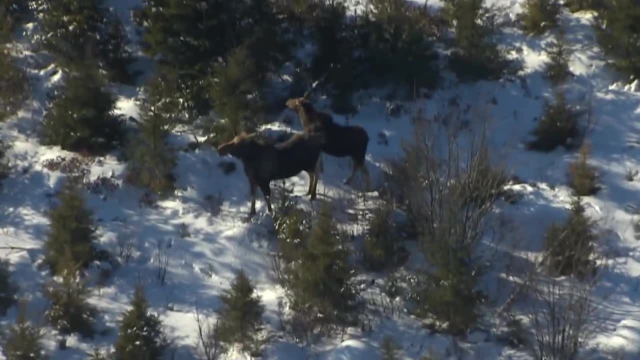 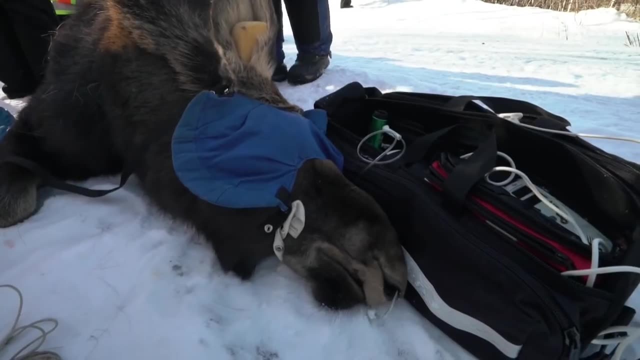 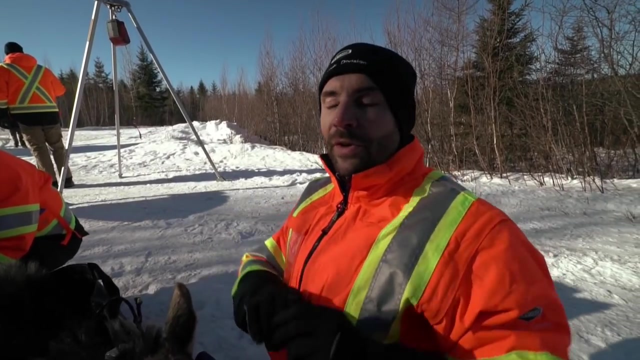 There's two right below us, straight to the right. A wildlife biologist uses a net gun to capture them. The net gun technique is very efficient, very safe for the animals. A vet is on hand to keep the animal comfortable. It's not really anesthetized, just sedation. We want her to be calm. 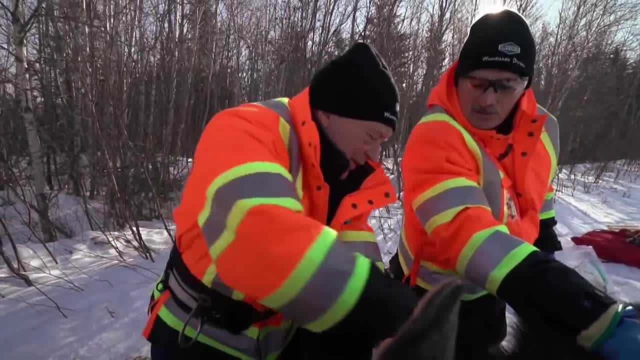 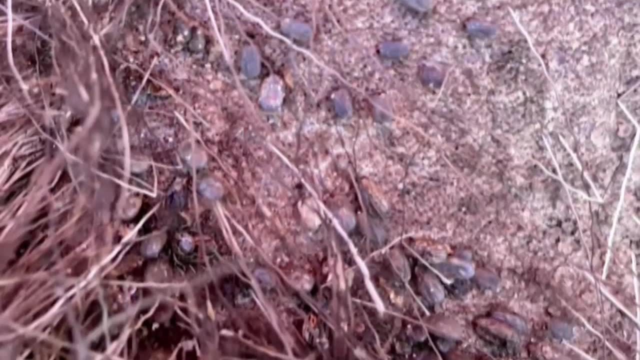 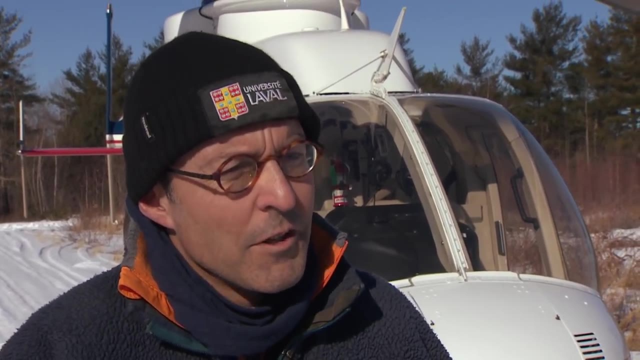 It allows the researchers to conduct their work. I'll start with the tick counter. This process gives them an idea of how many ticks are on the entire animal, literally sucking the life out of them. There's inflammation of the skin, They lose some of their fur and then they change their behavior. They use more of their time to groom. 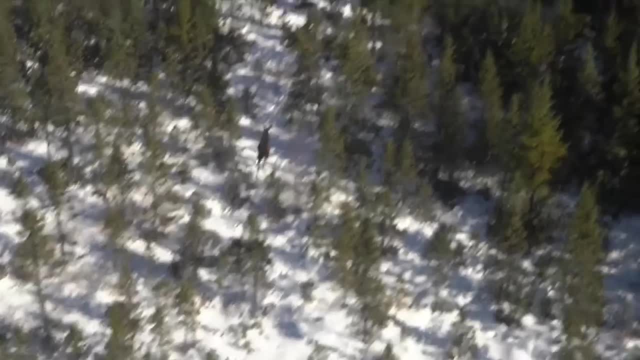 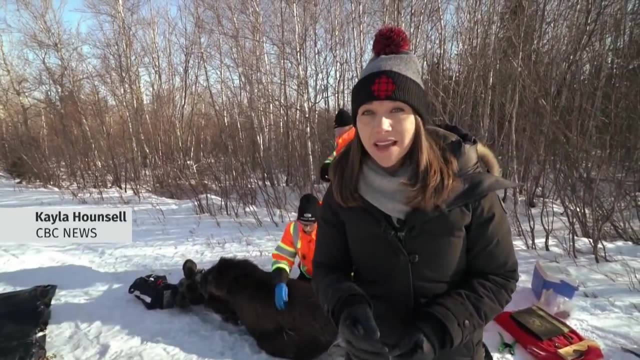 less of their time to eat. In nearby New Hampshire and Maine scientists have found up to 70 percent of moose calves have died during the winter. Up to 80,000 ticks have been found on a single moose, 80,000 on just one moose. Now these scientists are worried climate change. 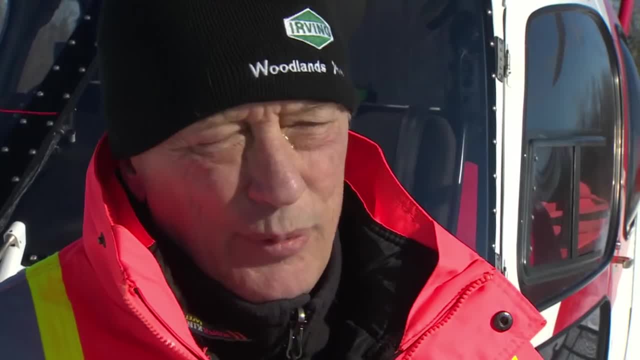 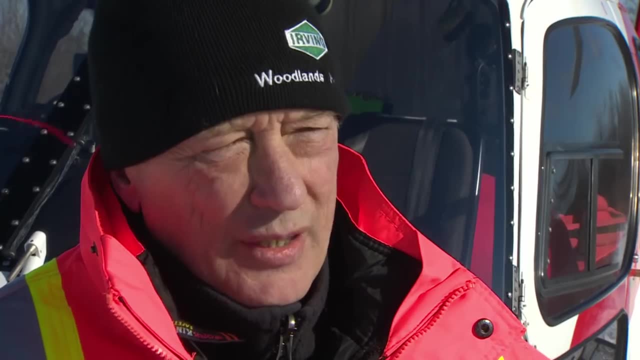 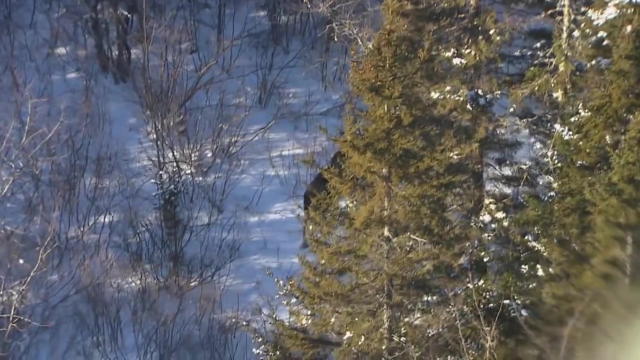 could be moving the same problem further north. The global warming is The global warming is The global warming is is likely increasing their abundance. The northern limit is moving north and north and north. Warmer winters and less snow cover make it easier for ticks to survive. 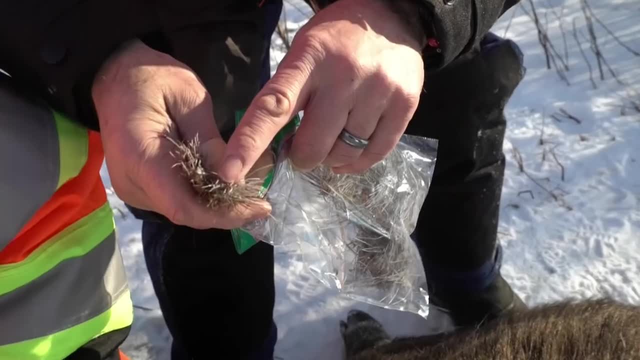 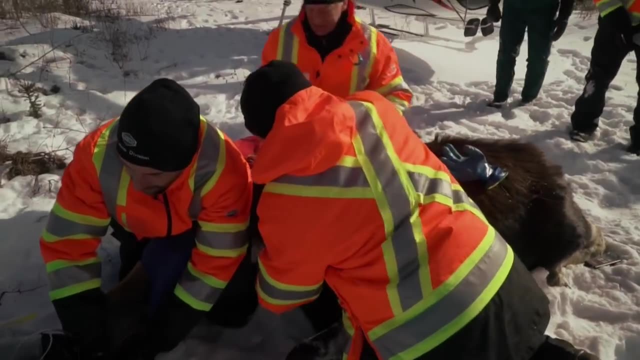 The scientists weigh the animal tag. it take a fur sample. They come out pretty easy. hey, Yeah, I'm at the place where the tick eats And give it a collar, Our GPS collars. we can control them remotely so we can get a location once every hour.